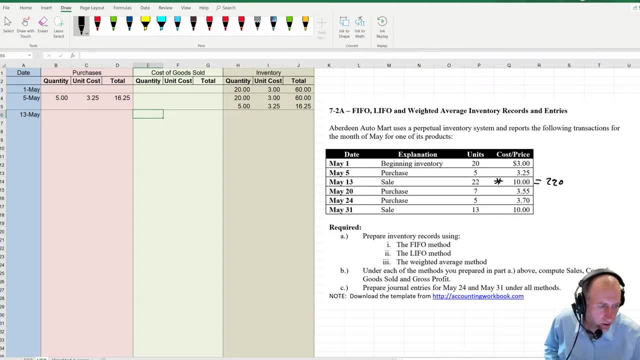 $220.. $220 times 10 is $220 in revenue. I'm worried about not my revenue but my cost of goods sold. So I have to say which of these 22 units sold, And with LIFO it's the newest or the most recently purchased stuff. So 5 sold. all of those sold, all those ones, and 17 of those gets me up to $22.. 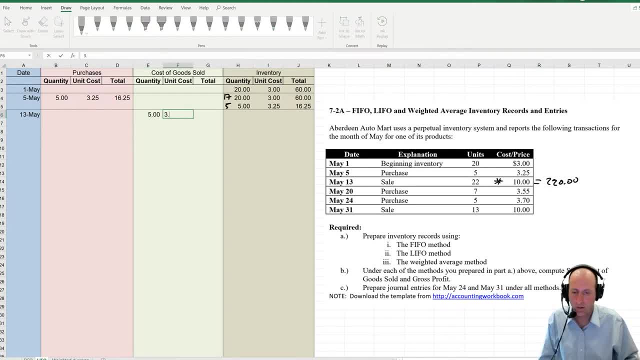 So I sold 5 at $3.25, and I sold 17 at $3. 5. 5. Times $3.25, and 17 times 3. What does that leave me with? It leaves me with 2 $3 units. 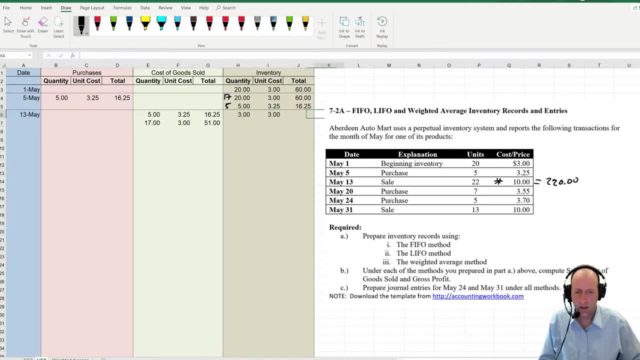 Or 3 $3 units. Pardon me, 3 left over 3 times 3 is 9.. Okay, So that's really the key item. Now we make a couple more purchases, May 20th. 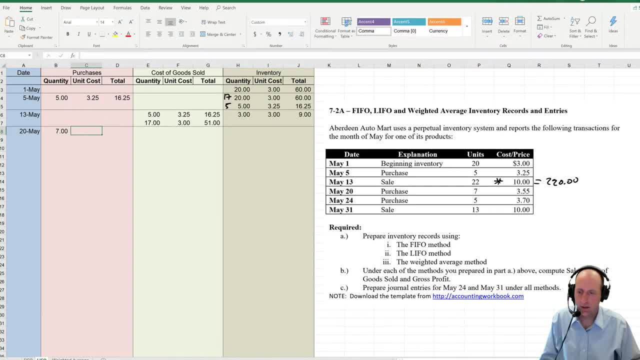 May 20th we buy 7, that costs $3.55,. equals that times that $24.85.. There's no cost of goods sold because we didn't sell any goods. So we had 3 at 3 for $9. 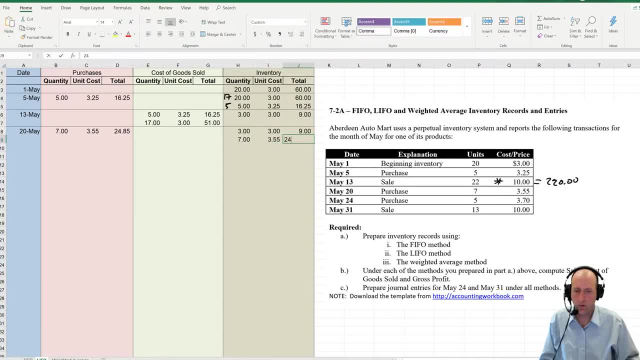 Now we're adding to it 7 at $3.55 for $24.85.. And that brings us to May 24th. We buy 5 more May 24th. we buy 5 at $3.70,. 5 times $3.70, is $18.50. 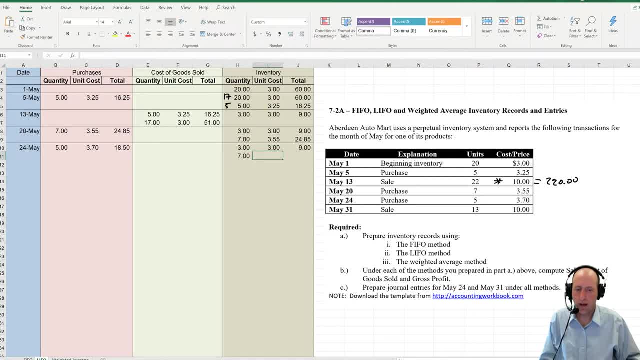 I had 3.. I didn't sell them, so I still got them. I had 7 at $3.55 for $24.85.. Again, I didn't sell them, I still got them. And now I'm adding to it 5 at $3.70 for $18.50. 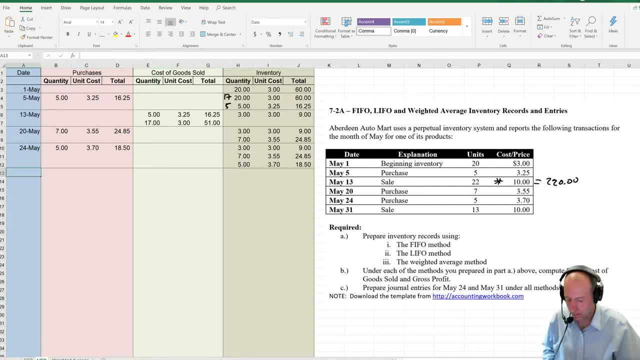 So that's May 24th. Now on May 31st, my mother's birthday, what happens? We sell 13.. We've got to say which 13 did we sell. We sold the most recently purchased 13.. 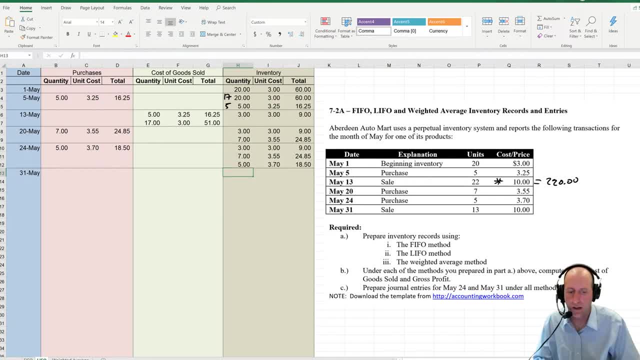 So we sold the. well, let's see, Just looking from bottom to top now, We must have sold all 5 of those. We must have sold all 7 of those. That gets us up to 12. And we must have sold 1 of those to get us to 13.. 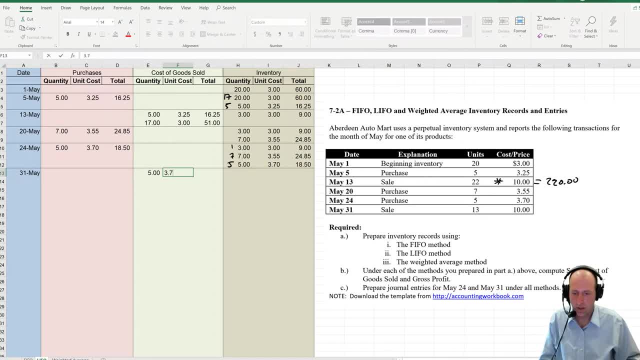 So, in order, I sold 5 for $3.70.. That's $18.50.. I sold 7 at $3.55.. 7 times 3, 55.. $24.85.. And I sold 1 at $3.00. 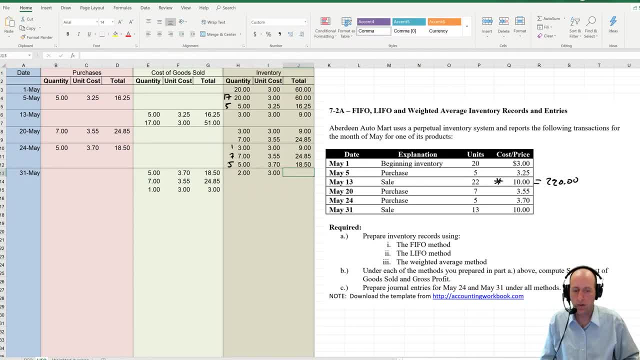 And I know 1 times 3 is 3.. Leaving me 2 at $3.00 for $6.00.. Put an underline under here And we are done with that part of the question. We have prepared our inventory record. 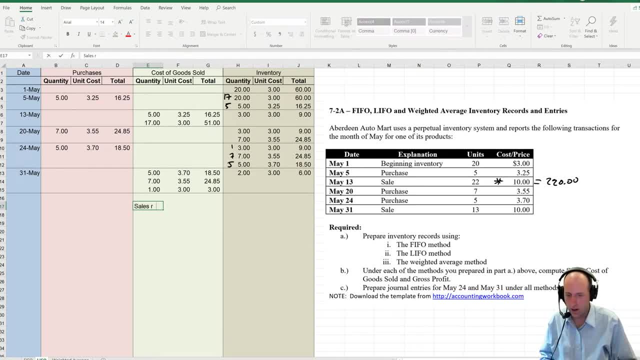 Now let's compute sales cogs And gross profit. Our sales revenue is just: we look on the sale date And we figure out how much we sold stuff for. So 22 times 10 is 220.. 5 times 3,, 70.. 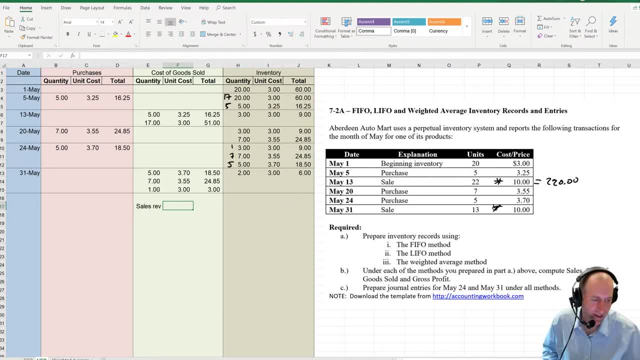 Oh wait, That's a purchase. 13 times 10 is 130.. So 220 plus 130, $350.. And this is the same across each method. So our sales rev is 350.. Our cogs cost a good. 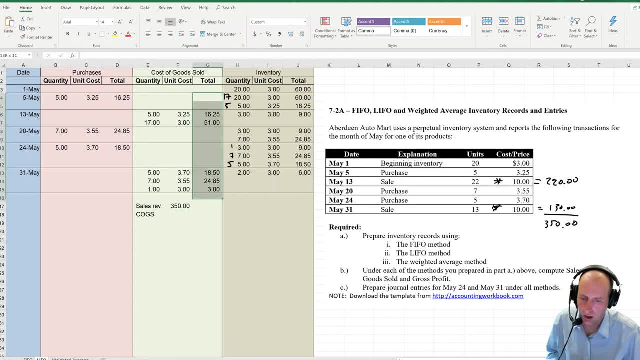 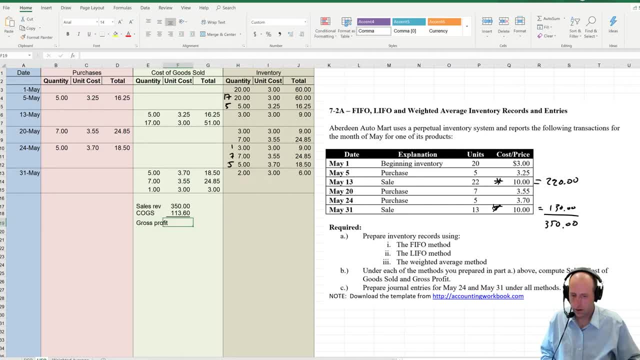 Sales minus cogs is gross profit. 350 minus 113 is 236.40.. So there we've answered B On to C. Journal entries should be very, Very straightforward. here we are doing journal entries just for May 24th and 31st we. 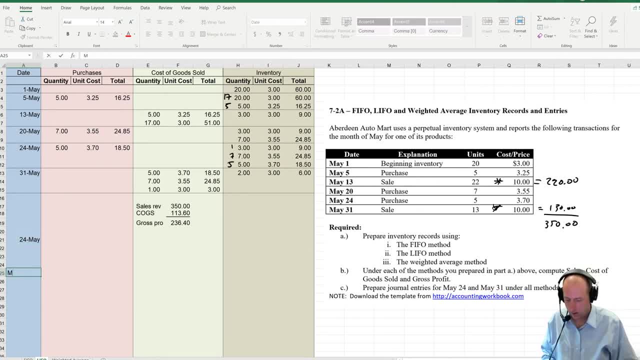 could be forced to do them all, but we're not here. so May 24th and May 31st: I know May 24th was a purchase, so when I'm buying inventory debit, inventory credit AP. and I know May 31st was a sale, so I know there's two parts to it: debit, AR or 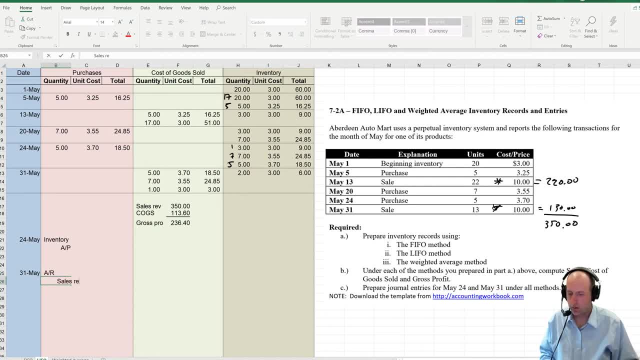 cash. it's unclear here: credit sales, rev, debit cogs, credit inventory. and now let's figure out our amounts. on May 24th, how much inventory did I buy? well, I bought $18.50 worth of inventory, just right here. I bought 1850, so debit.